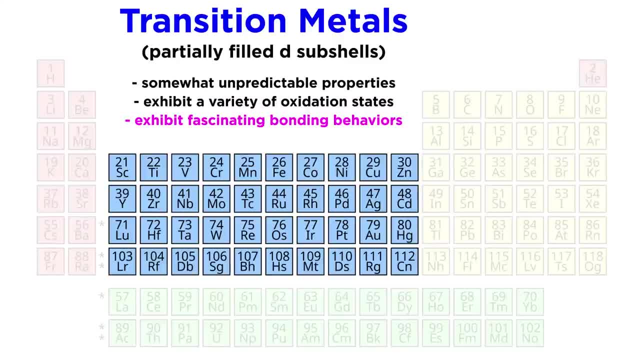 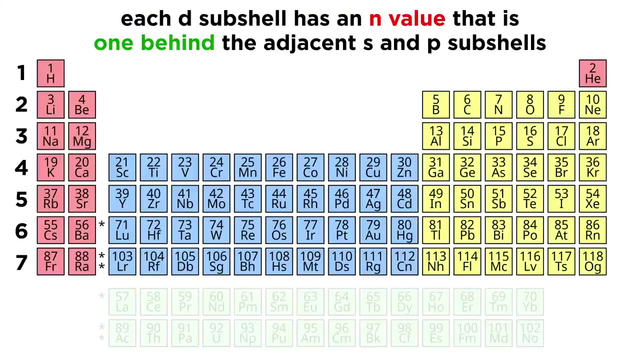 states and they have fascinating bonding behaviors, as we will learn progressively throughout this series. But these elements have an enormous range of applications beyond their utility in organometallic chemistry, which will be our primary focus. so let's talk a bit about these elements right now. One thing to keep in mind is that, because 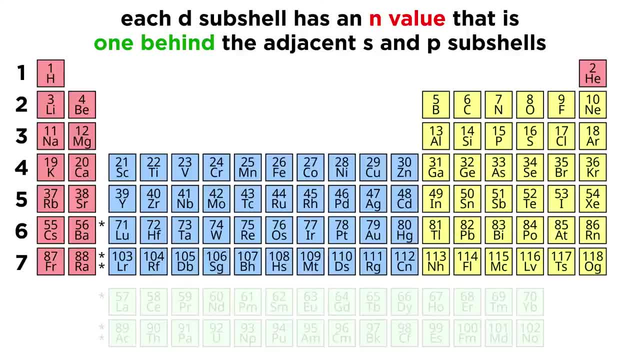 of the shapes and relative energies of the different orbitals. each period has a different D subshell that is one behind its S and P subshells in terms of principal quantum number. So the transition metals in the fourth period are filling their 3D subshell. those in the 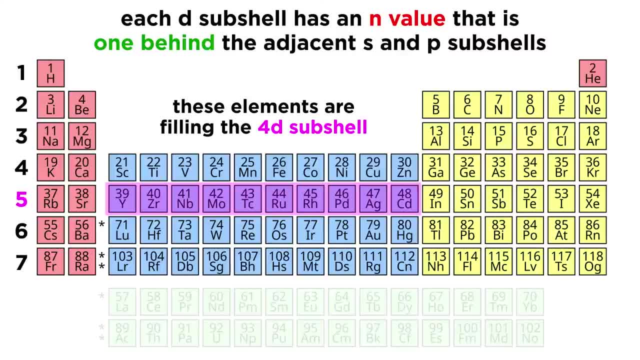 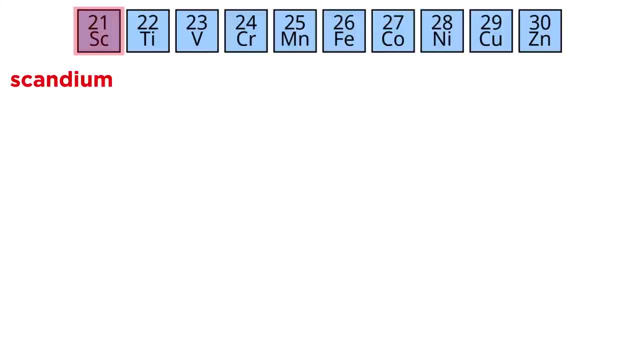 fifth period, are filling their 4D subshell and so forth. Let's start by looking at this first row of the D block. From left to right we have scandium, titanium, vanadium, chromium, manganese, iron and copper. 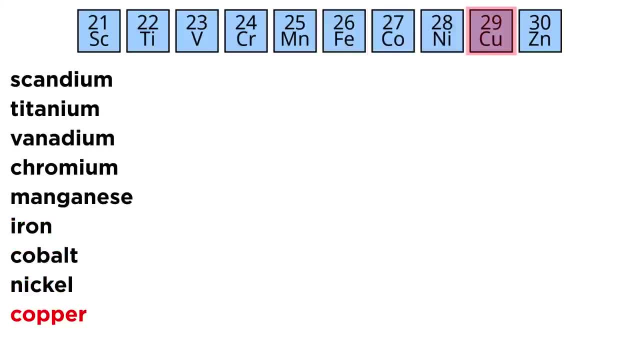 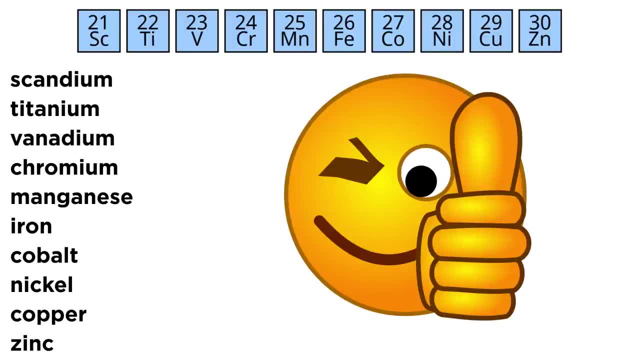 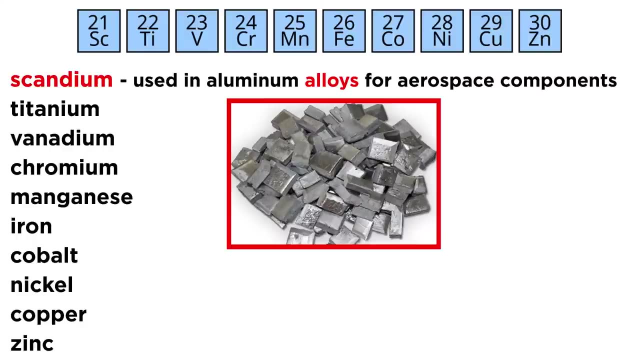 Cobalt, nickel, copper and zinc. Most of these should be relatively familiar, whether from their common use in everyday materials or from compounds we learned about in organic chemistry, while a few might be unfamiliar. Scandium is used in aluminum alloys for aerospace. 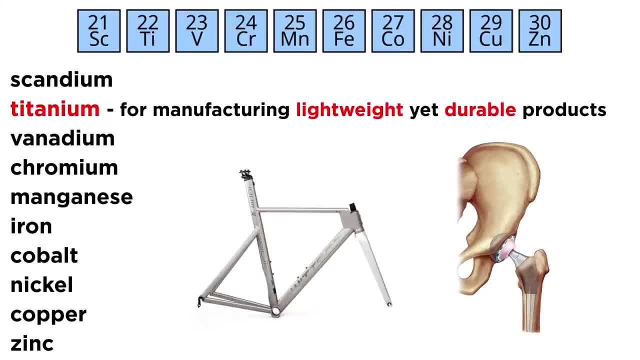 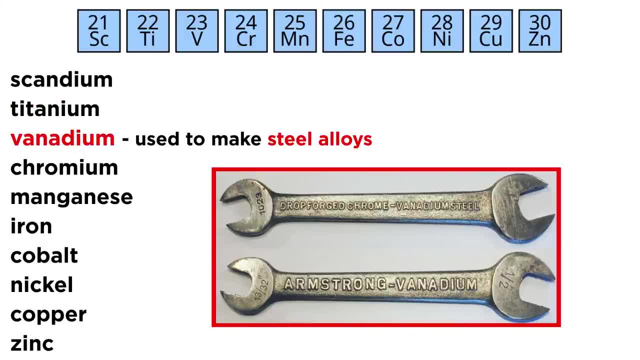 components. Titanium is an important metal for manufacturing lightweight yet durable products, from bicycle frames to artificial hips. Vanadium is used to make aluminum. Vanadium is an important metal for manufacturing lightweight, and it is used to make steel alloys. Chromium is used as a protective plating on plumbing. 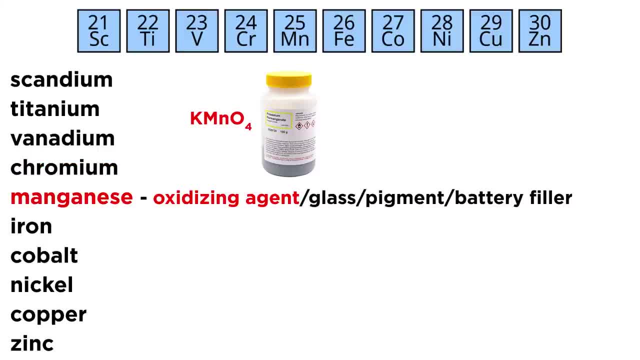 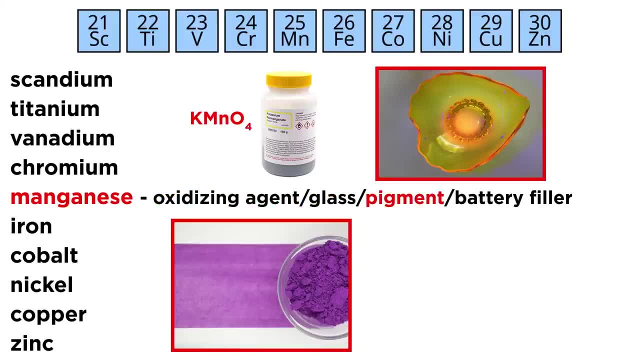 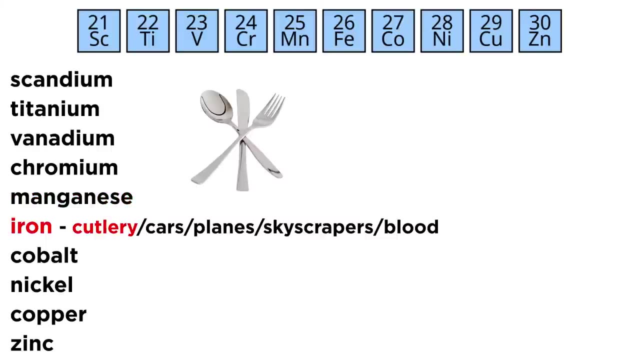 fixtures and automotive detailing. Manganese should be familiar from oxidizing agents like potassium permanganate. It is also used to make glass as a pigment and as filler in dry cell batteries. Iron is absolutely everywhere, from the cutlery in your kitchen to cars, planes and skyscrapers. 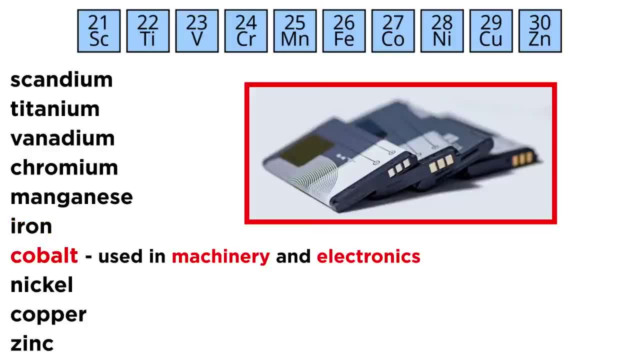 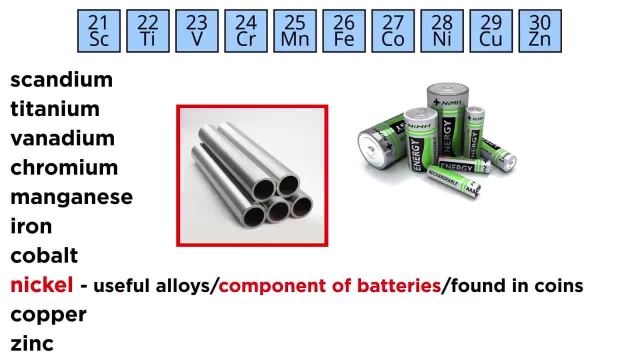 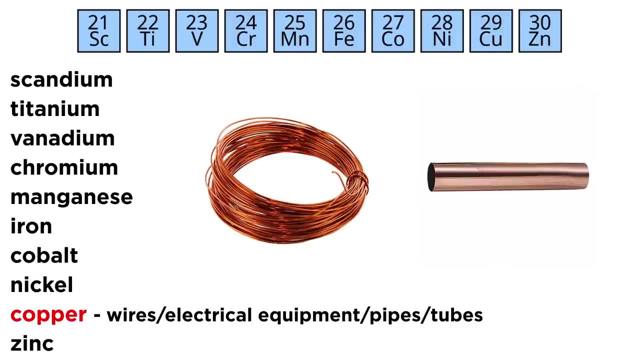 It's even in the hemoglobin in your blood. Cobalt is used in machinery and electronics. Nickel is found in useful alloys and is an important component of many batteries. It is also used to make coins. Copper is tremendously useful for making wires and other electrical equipment, as well as pipes and tubes, And 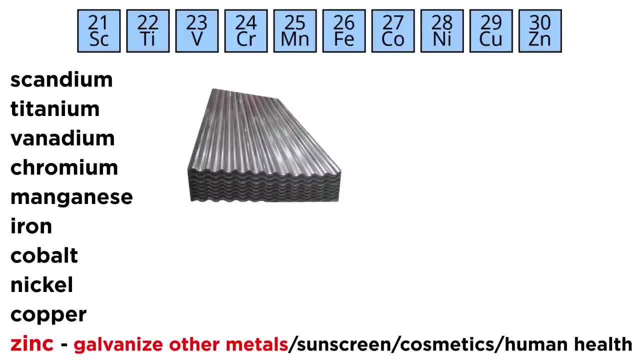 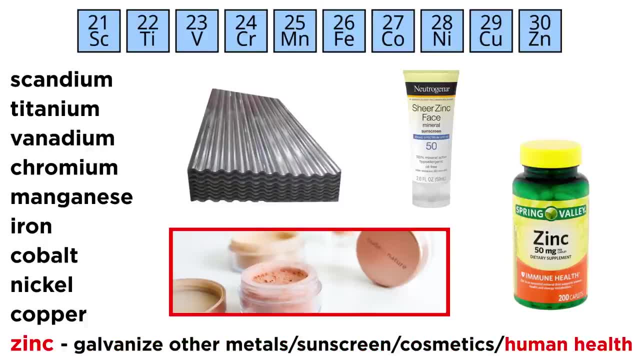 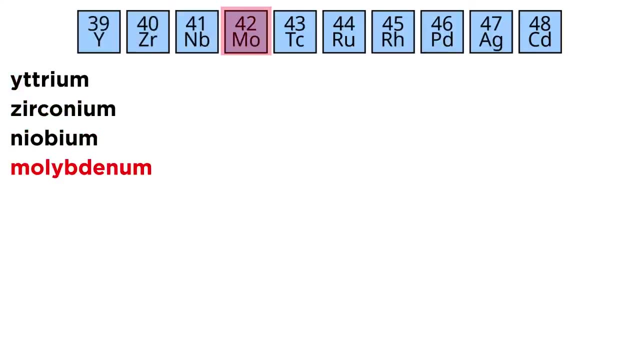 zinc is frequently used to galvanize other metals to prevent rusting. It is also used in sunscreens and cosmetics and is essential to human health. Thanks for watching. Have a great day, Bye. Moving on to the next row, we have yttrium zirconium, niobium, molybdenum technetium. 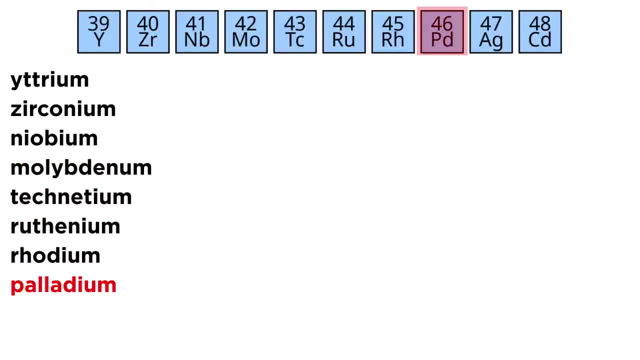 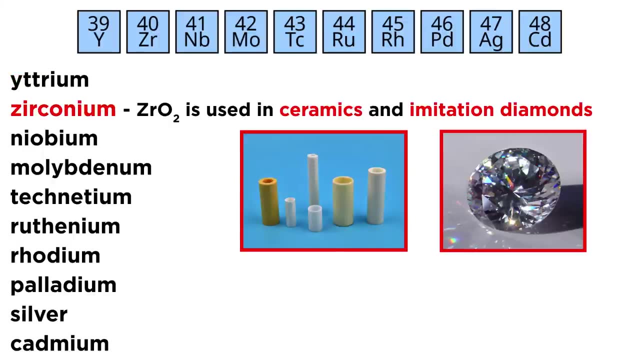 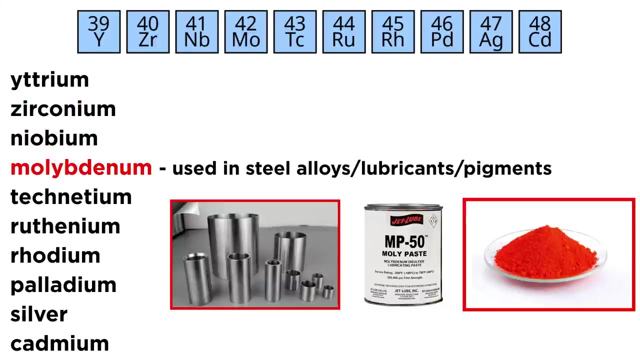 ruthenium, rhodium, palladium, silver and cadmium. Yttrium is found in aluminum and magnesium alloys. Zirconium oxide is used to make highly durable ceramics, as well as imitation diamonds. Rhodium is used in various alloys and superconducting materials. Molybdenum is used to make steel. 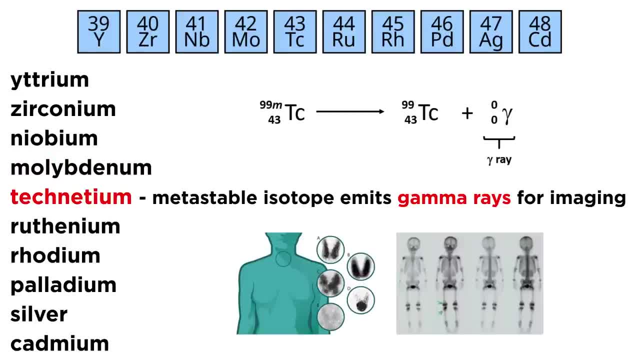 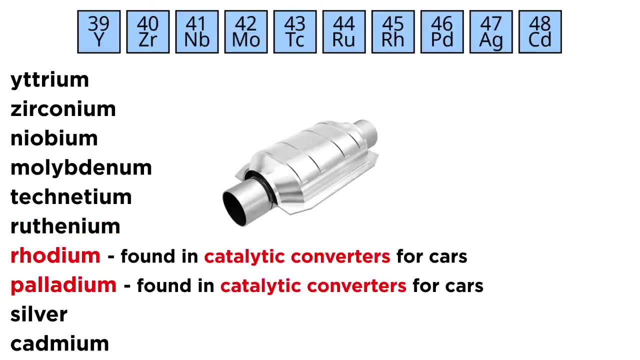 alloys, as well as lubricants and pigments. Technetium has an isotope that is metastable and emits gamma rays that give it utility in medical imaging. Ruthenium oxide is used to coat electrodes. Rhodium is used in catalytic converters for cars, as is palladium, Silver. 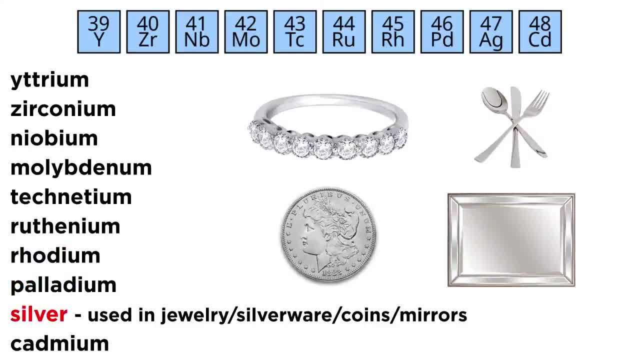 is used to make jewelry and silverware. Zirconium is used to make jewelry and silverware. Rhodium is used to make jewelry and silverware. Zirconium is used to make jewelry and silverware. Rhodium is used to make jewelry and silverware, Silverware, coins, as well as mirrors, being that it is. 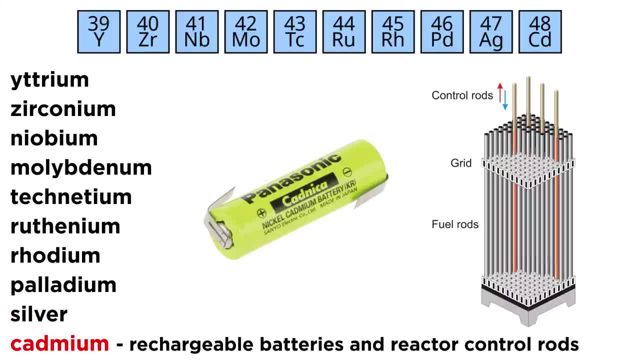 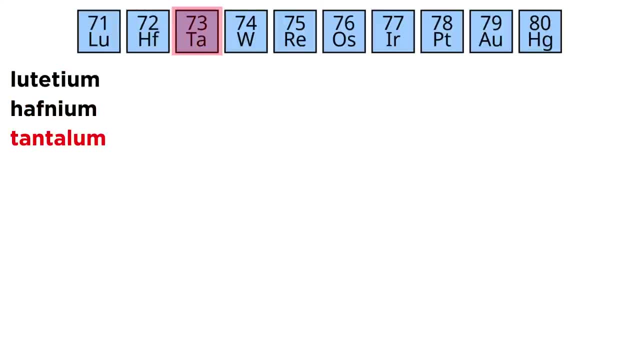 the best reflector of visible light we know of, And cadmium is widely used in rechargeable batteries as well as control rods for nuclear reactors. Arriving now at the third row, in this block we find lutetium, hafnium, tantalum, tungsten. 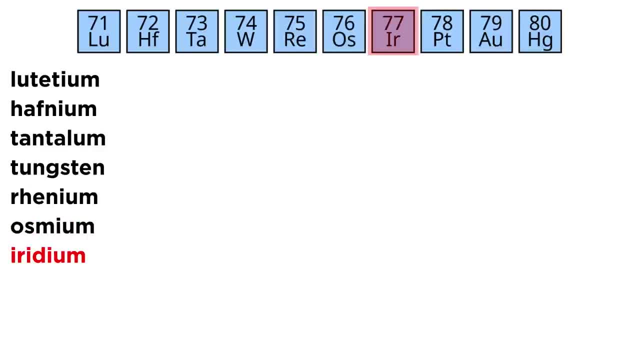 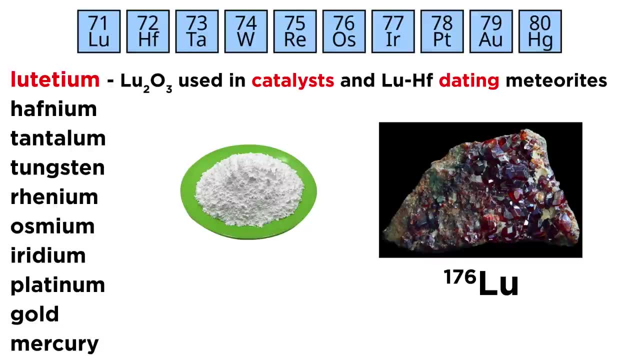 rhenium, osmium, iridium, platinum, gold and mercury. Lutetium oxide is used to make catalysts in the petrochemical industry, and lutetium-hafnium dating is used for determining the age of meteorites, due to the long half-life of lutetium-176.. 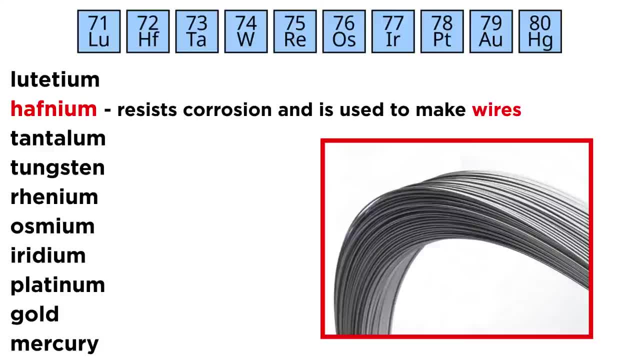 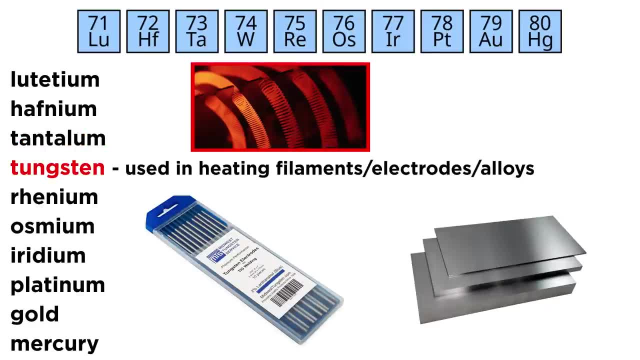 Hafnium resists corrosion and is used to make wires. Tantalum is also used to make wires and is present in various alloys. Tungsten is widely used in heating filaments as well as electrodes and is present in many useful alloys. It has the highest tensile strength. 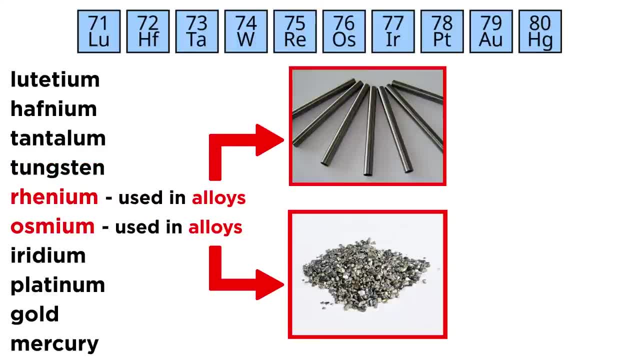 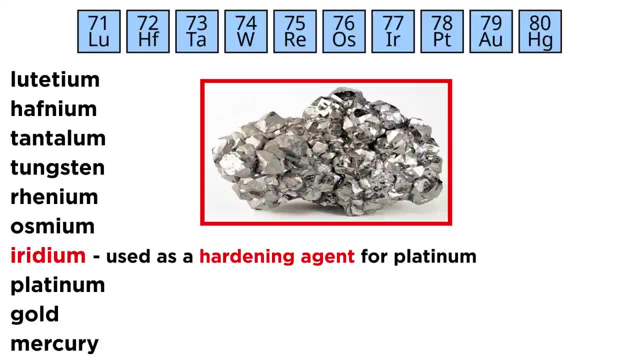 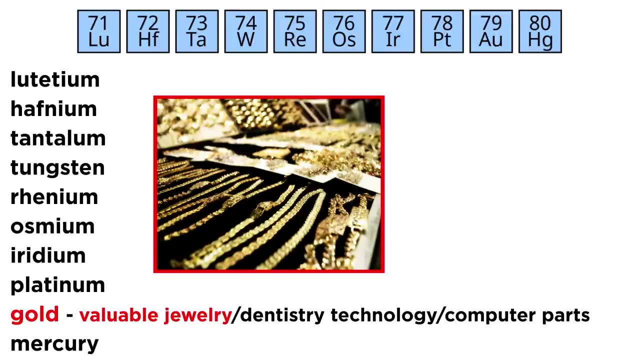 and melting point of any element. Rhenium and osmium are primarily used in alloys. Iridium is used as a hardening agent for platinum, which is used in jewelry, electrodes and other laboratory instruments. Gold is famous for its monetary value and is used in jewelry. 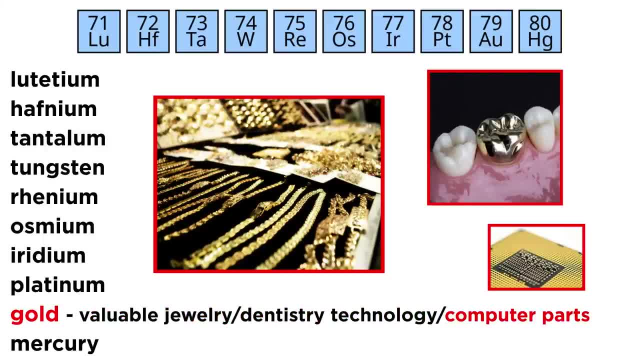 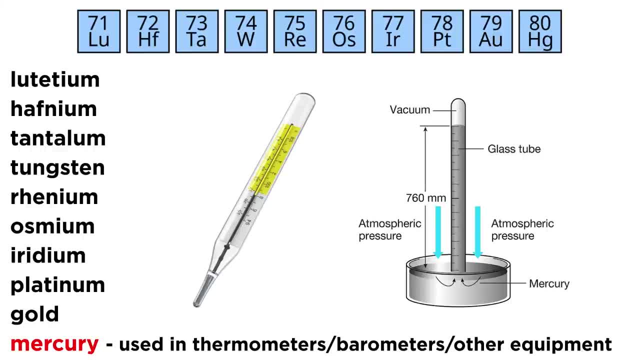 for this reason, but is also important in dentistry and silverware. Gold is also used in certain computer components, And mercury has long been used in thermometers, barometers and other scientific instruments, although due to its toxicity was eventually disfavored. 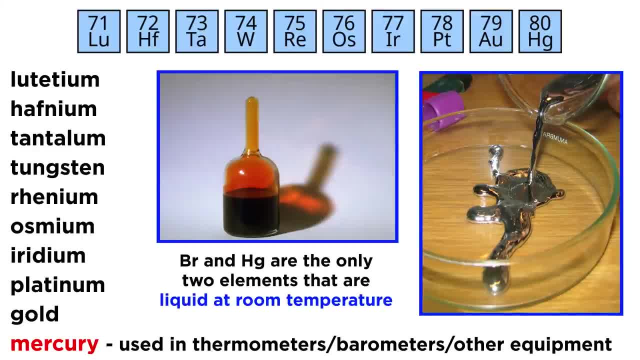 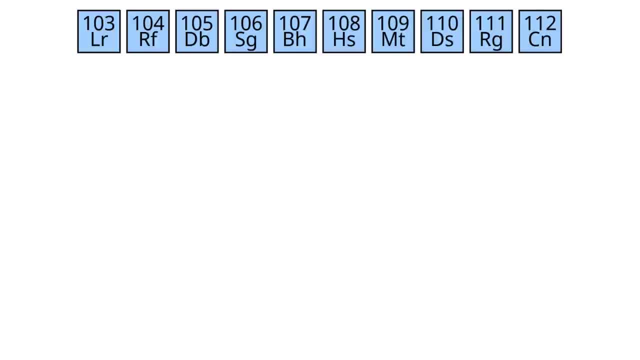 for other substances. As we already learned, mercury is one of only two elements, along with bromine, that is liquid at room temperature. And finally, the fourth row in the block, which is part of period seven, includes lorencium. 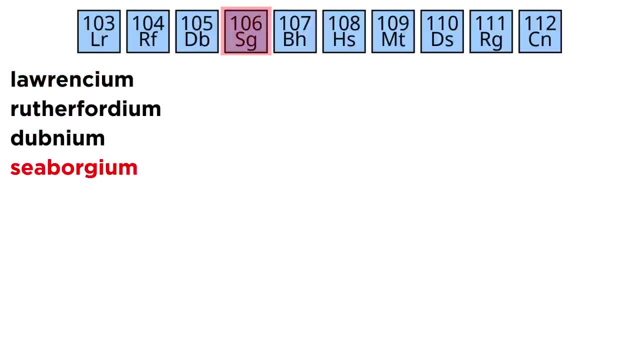 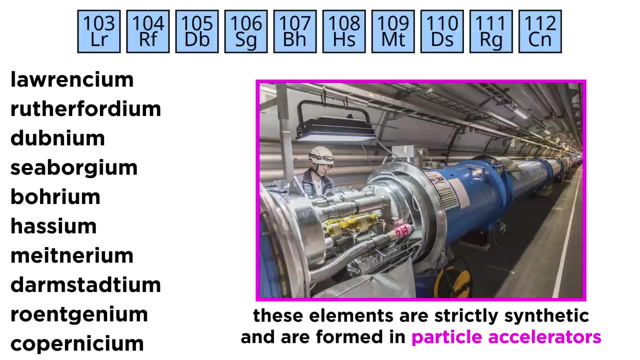 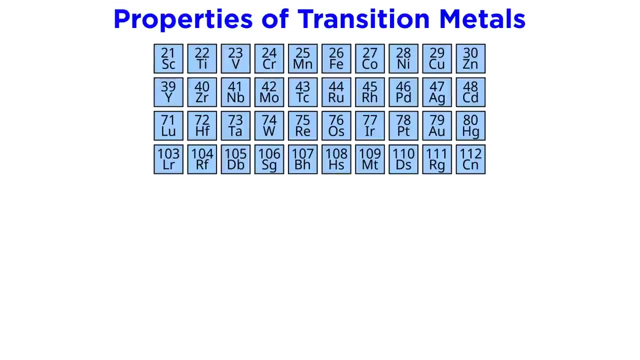 rutherfordium, dubnium and lutetium. None of these elements occur naturally and are exclusively synthesized in particle accelerators, with only a few atoms having ever been made for most of these elements. They are all highly radioactive and have no application beyond scientific research. So what are some of the 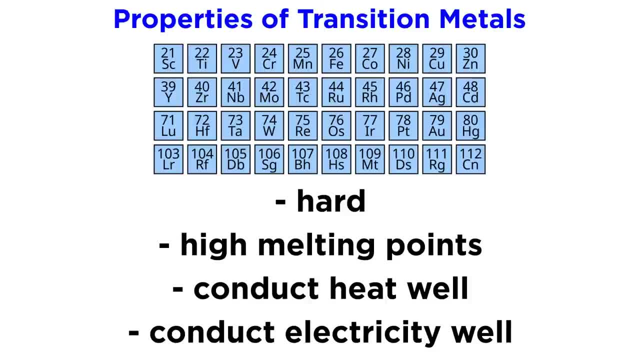 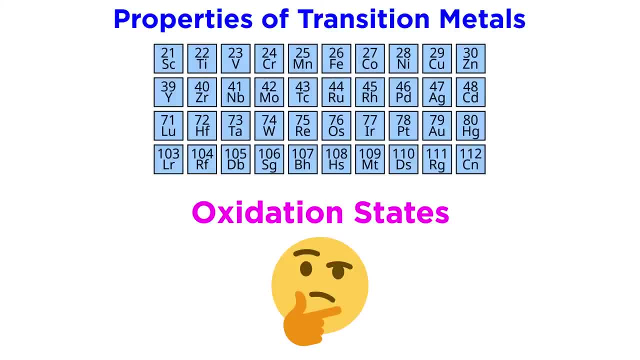 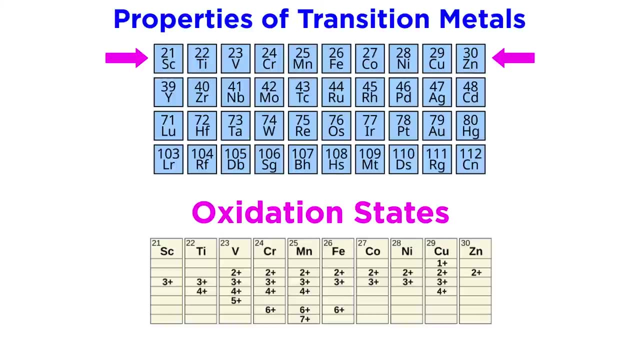 properties of transition metals. Most of them are hard, high-melting solids that conduct heat and electricity very well. One important thing to discuss is the common oxidation states of these elements. Here is a table illustrating the common oxidation states for the first row of the D block. As we can see, some elements like scandium and zinc have only one oxidation. 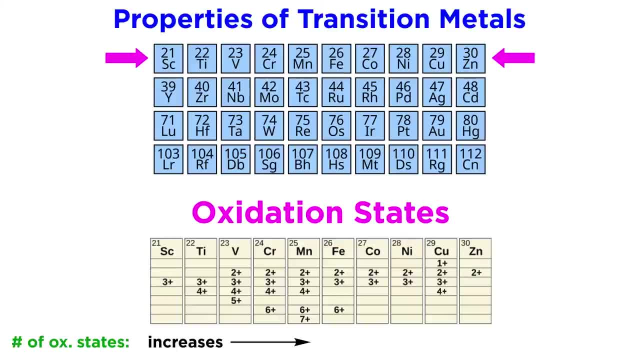 state, whereas manganese has five, and in fact, the number of possible oxidation states increases, moving to the middle of the table and then decreases to the end, apart from copper, which has at least four oxidation states. This is because, on the left side, 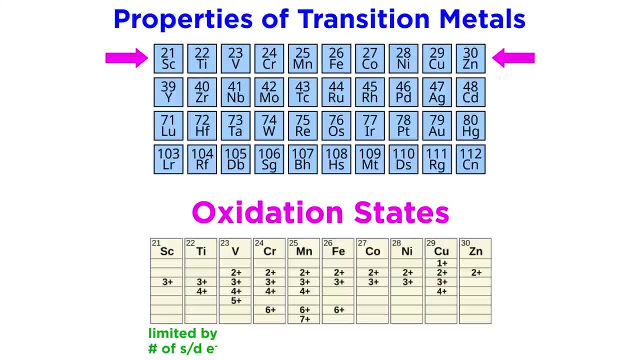 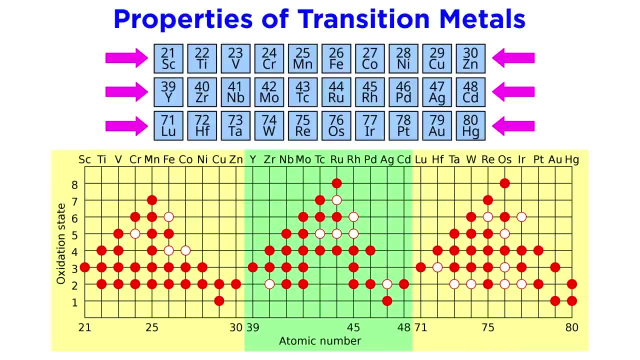 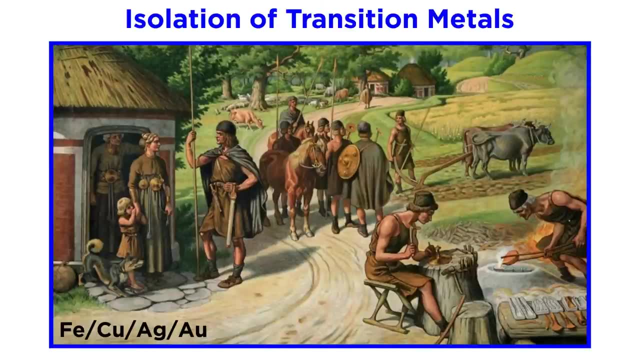 the oxidation states are limited by the number of electrons in the 4s and 3d subshells. Moving down to other periods, higher oxidation states become more and more common for reasons of increasing atomic radius In terms of isolating these metals, some of them have a very long 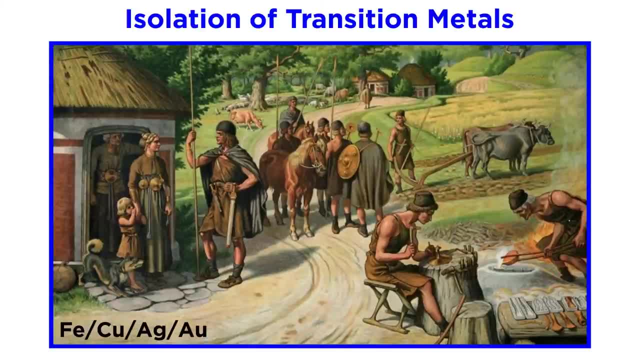 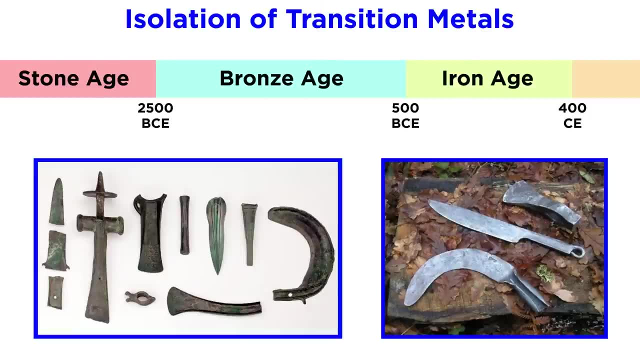 history as iron, copper, silver and gold have been known for most of human civilization. In fact, we demarcate certain periods in human history as the bronze age and iron age to indicate when we became able to isolate certain metals and use them to make tools, weapons. 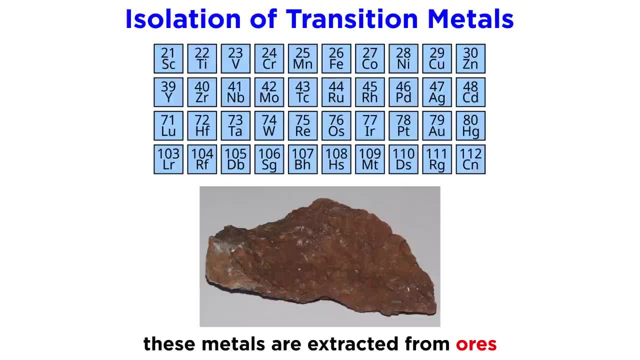 and other things. Most of the other transition metals are extracted from various ores, which present a range of difficulty depending on the metal's concentration, The transition metal's concentration, what else is present in the ore and ease of reduction to the neutral. 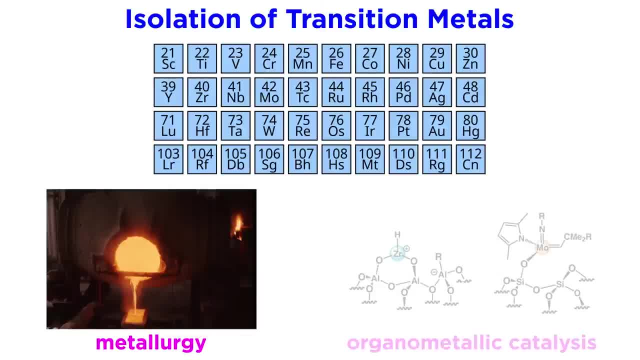 metal. But as the goal of this series is less of a focus on metallurgy and more on organometallic catalysis, we will not discuss the details of this process for each individual metal. Instead, we just want to get a general sense of their properties. as certain metals will. 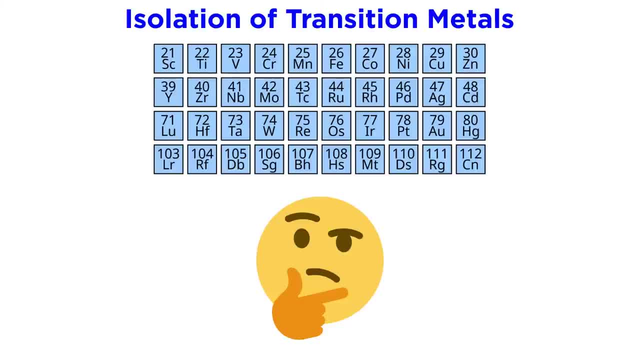 come up again and again as we learn about different reagents and catalysts. With the D block covered, there is just one second to the next. So let's get started. With the D block covered, there is just one second to the next, as certain metals will. 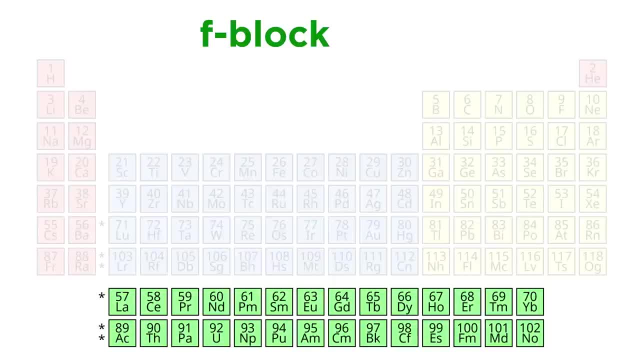 come up again and again as we learn about different reagents and catalysts. With the D block covered, there is just one section of the periodic table left, and that's the F block. This is always found hovering mysteriously below the rest of the table, and this is for. 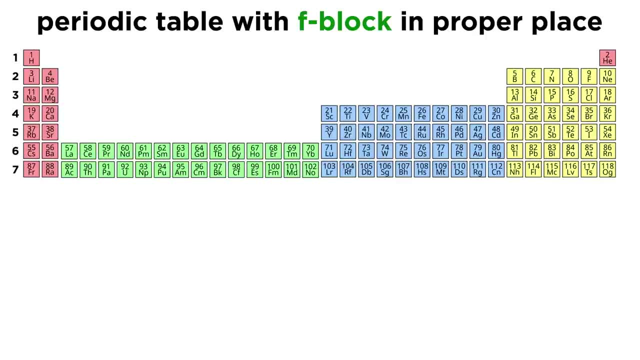 very good reason. If the periodic table were to be displayed intact, the F block would occur immediately after the S block in periods 6 and 7.. So that would look like this, with the S, F, D and P blocks in this order, so that there is no interruption in the increase. 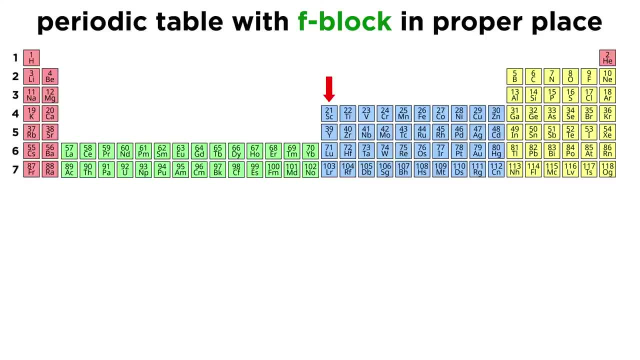 of atomic number when moving left to right up. The only thing is that scandium and yttrium should actually shift over to sit above lanthanum and actinium because they have similar electron configurations ending in D1. This may seem a bit confusing, but it is only after one D electron is present that the F 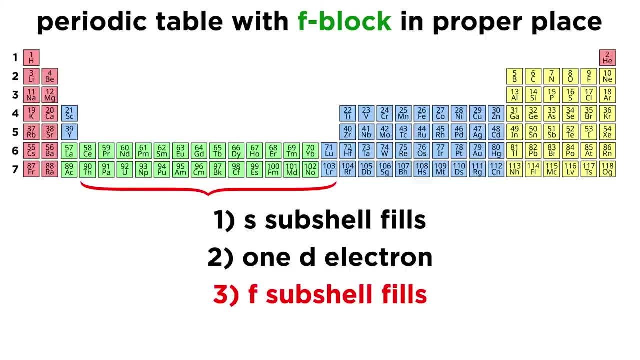 subshell begins to get filled, so the rest of the F block comes next, and then only once we get to this column with hafnium and rutherfordium do elements begin adding D electrons again, even though the D block technically begins one group sooner. 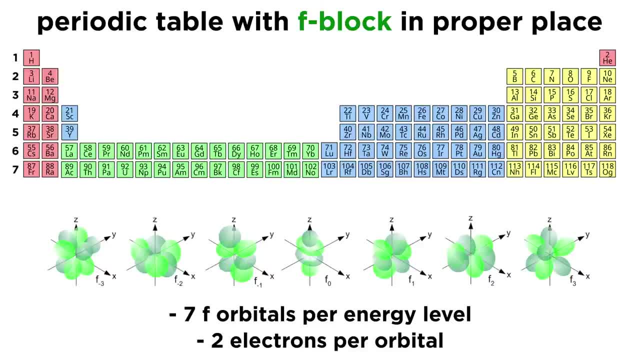 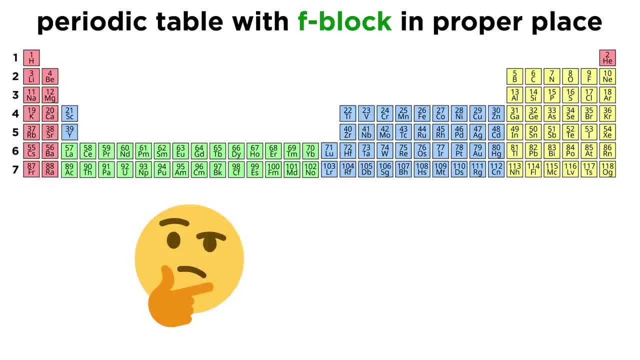 At any rate, since there are seven F orbitals per energy level, the F block is fourteen elements long, And because we almost never have to discuss any of these incredibly rare elements, except for maybe uranium from time to time, it is much more convenient to snip this region out. 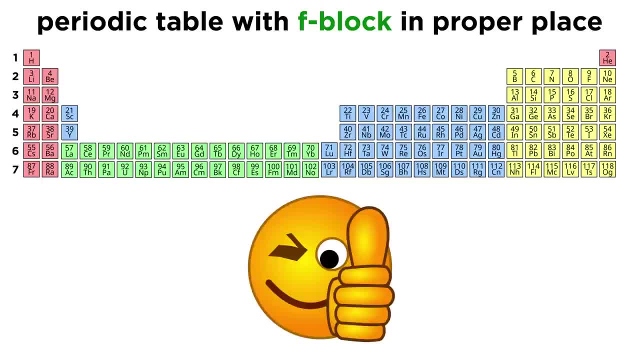 and condense the rest to make it more manageable. But it is very important to note that this is where the F block would go if all the elements were to be displayed continuously, Much like with the D block, because of the shapes and relative energies of the orbitals. 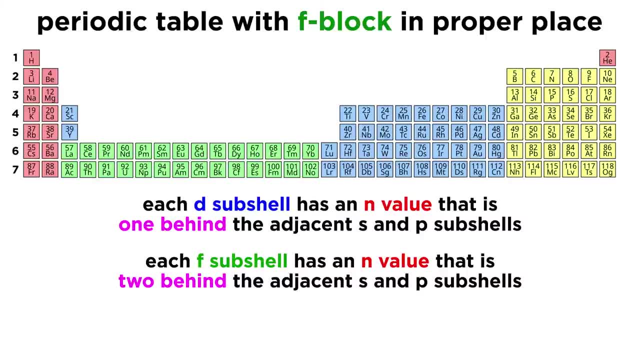 the F subshell for a given period will be two behind the S and P subshells and one behind the D subshell in terms of principal quantum number. So period six goes six S, then four F, then five D, then six P, While period seven goes. 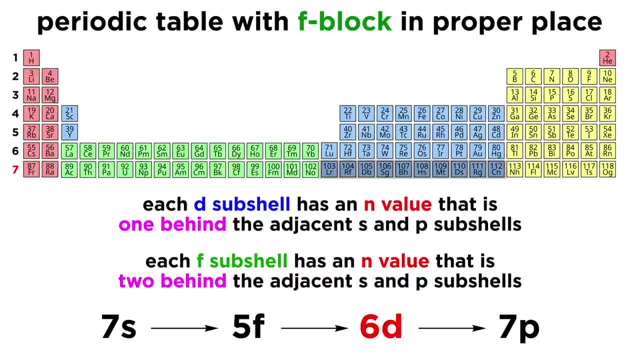 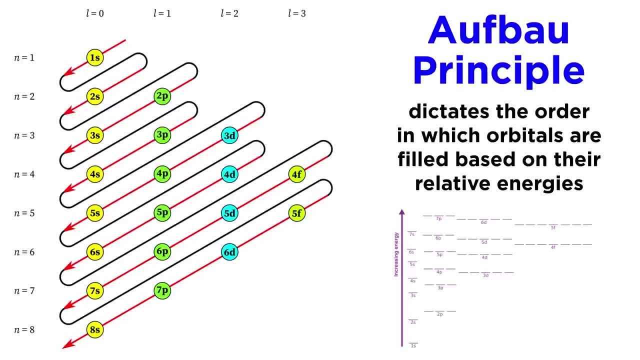 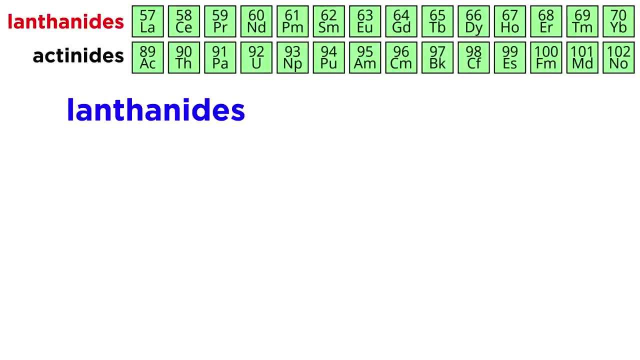 seven S, then five F, then six D, then seven P. This is strictly due to the Aufbau principle, which dictates the order in which orbitals will be filled. Let's quickly go through and name these elements as well. The first row in the F block is called the lanthanides. 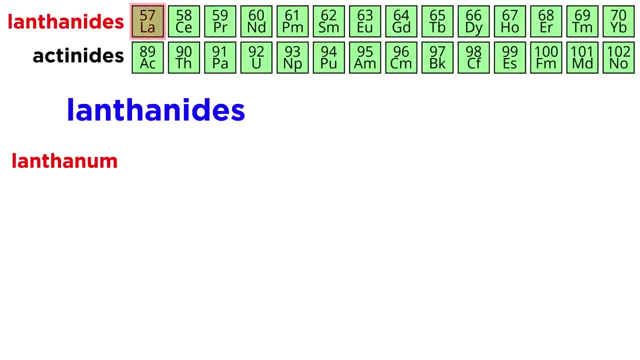 This is because the first element in this row is called lanthanum. After that we have cerium, praseodymium and praseodymium. The first element in this row is called lanthanum, After that we have cerium, praseodymium and praseodymium. 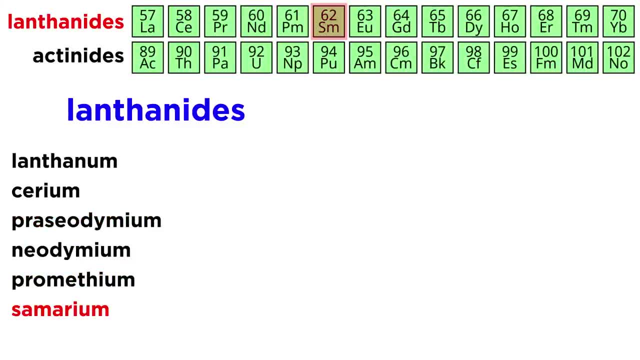 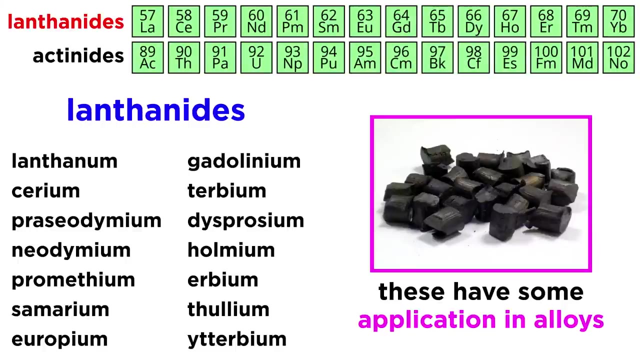 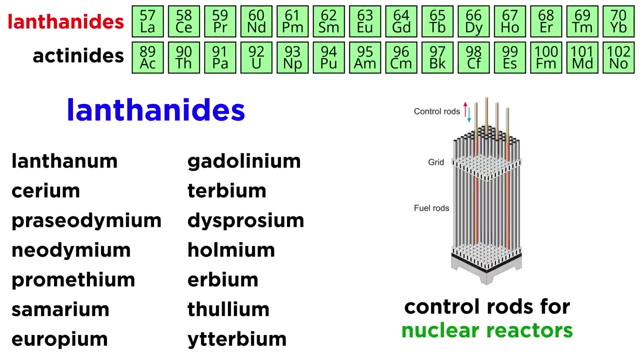 The lanthanides are still small and stable enough for some of them to have practical applications, primarily in alloys. But additionally, neodymium glass is used to make lasers and others are used in control rods for nuclear reactors. Then, finally, the second row in the F block is called the actinides, because the first 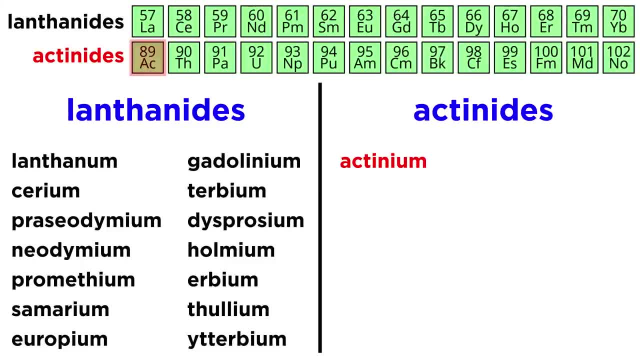 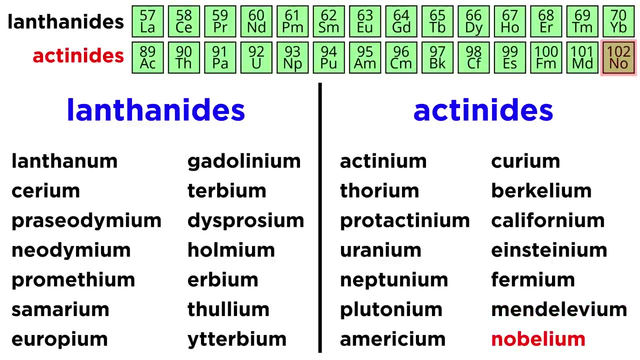 element in this row is called actinium. After that we have thorium, protactinium, uranium, neptunium, plutonium, americium, curium, berkelium, californium, einsteinium, fermium, mendelevium and nobelium.